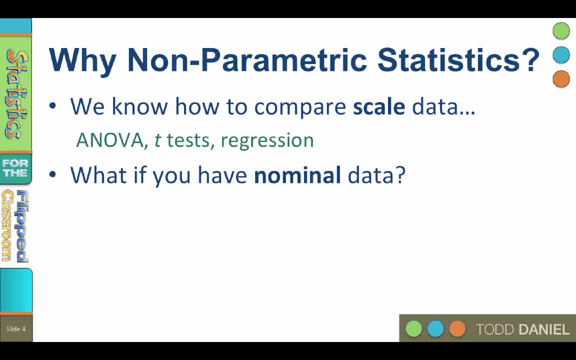 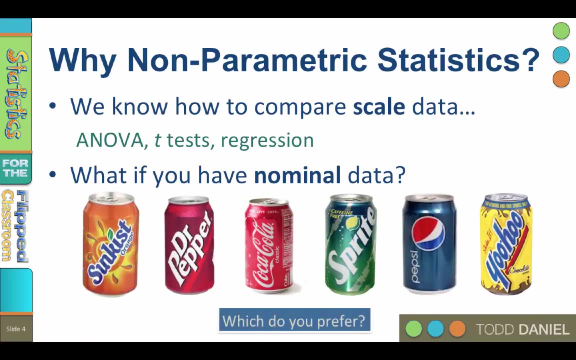 suggests that we just buy a case of whatever is on sale, because people will drink whatever is available. But you think that maybe people prefer one brand over others. So you offer the class a choice of six brands of soft drinks and ask everyone to choose their favorite. But how are you going to? 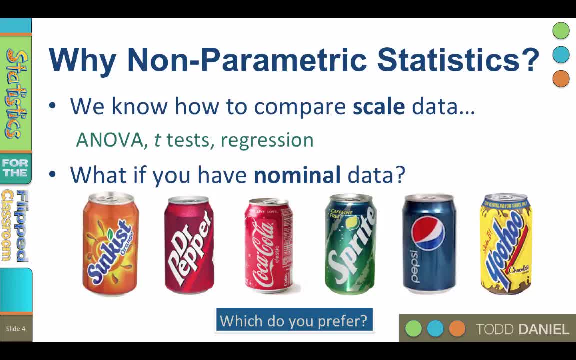 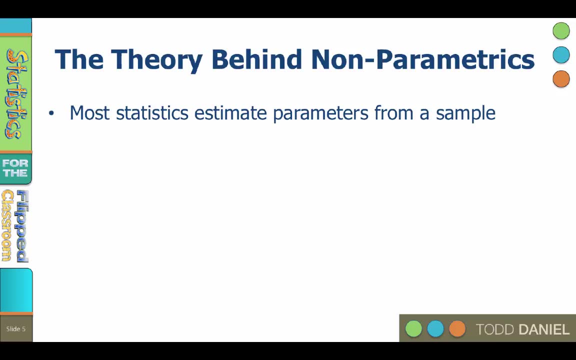 analyze these data? How can you tell if people truly have a preference for one type of soft drink or if they're simply choosing one at random? Most of the statistics that we have used so far estimate population parameters from a distribution of scores in a sample. So, for example, the t-test uses 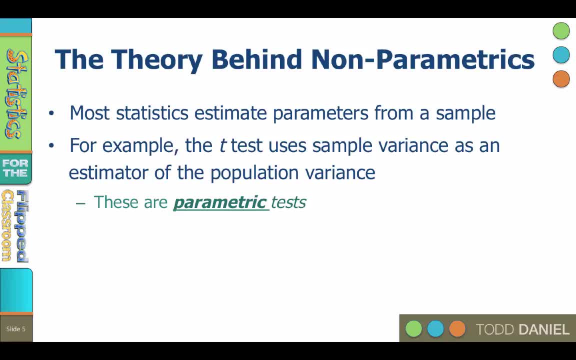 sample variance as an estimator of population variance. Tests like this are called parametric tests and they work because the central limit theorem shows us that the distribution of sample means will form an approximately normal distribution. But there is a class of tests that do not rely upon parameter. 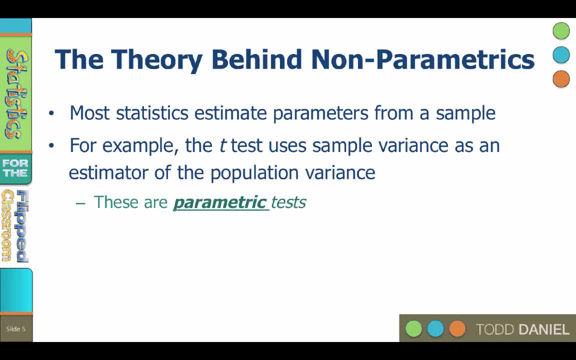 estimations or distribution assumptions, and these are called nonparametric statistics. Nonparametric are especially useful with nominal and ordinal level data, although they can be used with interval and ratio level data as well. So, for example, you want to make a comparison about whether males or 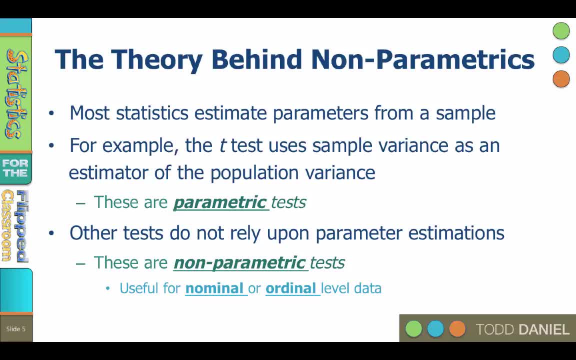 females are more likely to help a person in either emotional distress or physical peril. Or perhaps you want to know if patterns of soft drink consumption are the same at a state university as at a private school. Maybe you want to know if certain dormitories are over-represented or under-. 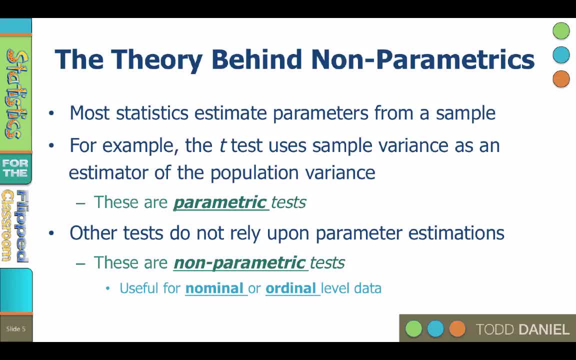 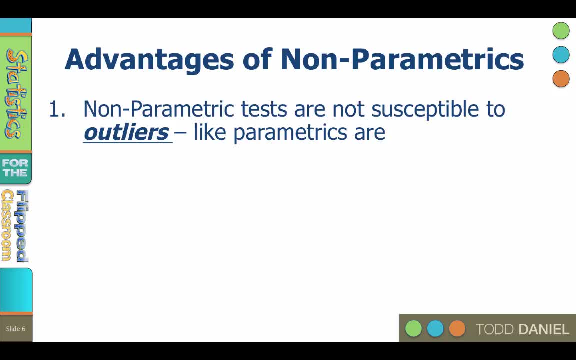 represented in their number of student government representatives. Nonparametric statistics have several advantages over paramedics. For example, if a student has a high score over parametric statistics, Number one: nonparametric tests are not susceptible to outliers, the way that parametric tests are One outlier score. 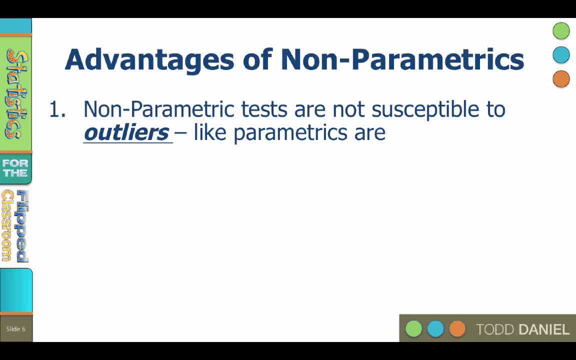 can affect a parametric test by inflating the variance and hence the error term. This can invalidate a conclusion drawn by the parametric test. so you make a type one error or perhaps even a type two error. Outliers in correlation can change the direction or the strength of a relationship between: 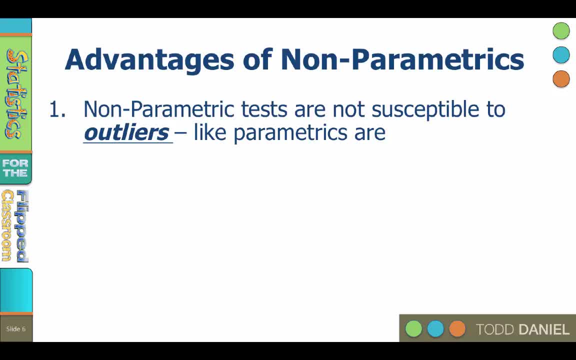 variables. But non-parametric tests do not have this limitation because they measure central tendency using ranked data. Ranking uses the median rather than a mean. So, for example, if the tenth number in your distribution is an outlier, that outlier can really shift the mean when you add it to other. 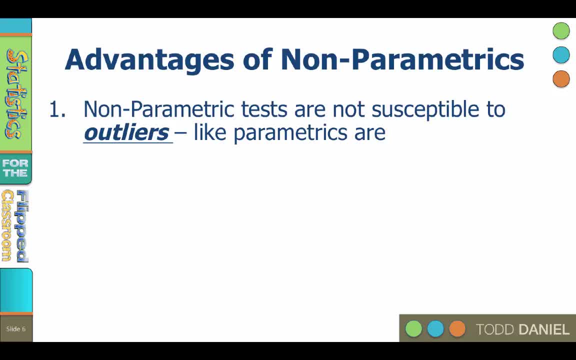 numbers, But when you are considering ranks, it is still just the tenth number, no matter how big the actual value is. So the main advantage of non-parametric statistics is that they do not require restrictive assumptions about the distribution. For instance, they do not assume that soft drink consumption is. 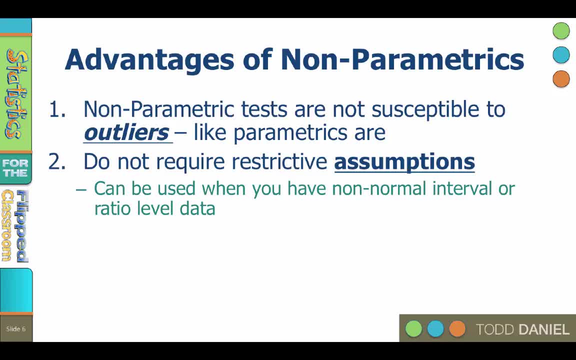 normally distributed. Non-parametric tests can also be used when you have non-normal interval or ratio data, such as data that are highly skewed. Typically, therefore, non-parametric statistics are only used when the data are too skewed to use a parametric test. 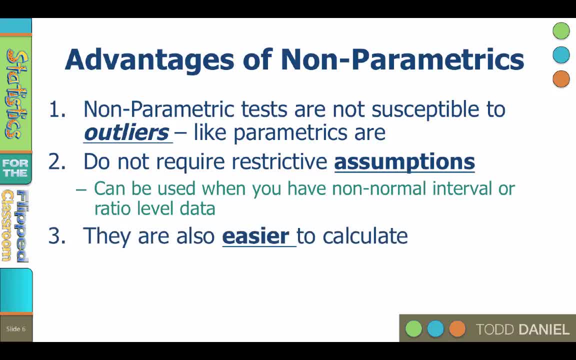 Another advantage is that non-parametric statistics are typically easier to calculate by hand, and we will practice doing some of them by hand in order to learn them. However, the main disadvantage of non-parametric statistics is that they are not as powerful as non-parametric statistics. They are not as powerful as non-parametric statistics. 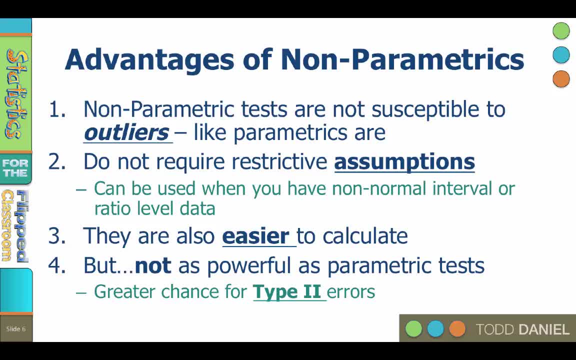 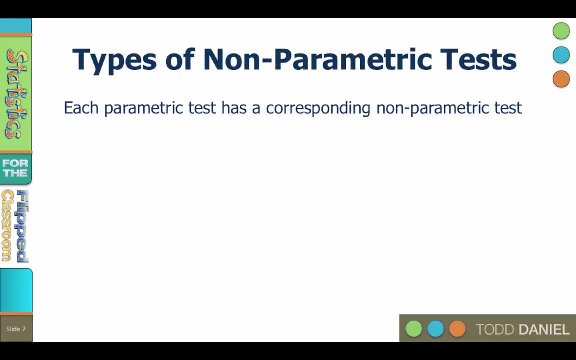 They are not as powerful as parametric tests. That means that they are more likely to miss an effect that truly exists or that you make a type 2 error. So as you get better with statistics, you will be using mostly parametric statistics, But you should keep some tools in your back pocket that you can. 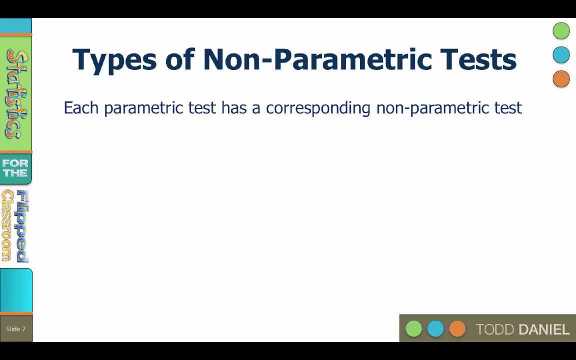 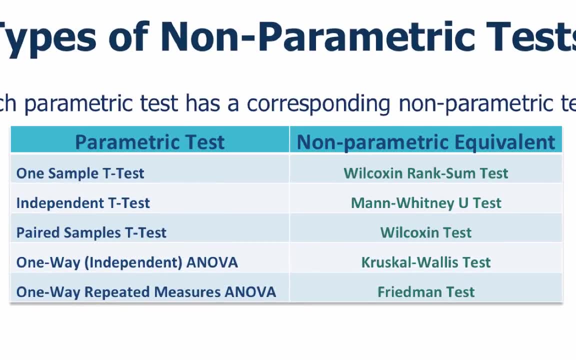 use. at times that the parametric statistics fail, Each parametric test has a corresponding non-parametric test. Here you can see each parametric test and its corresponding non-parametric alternative. So, for example, if you plan to do an independent samples t-test but